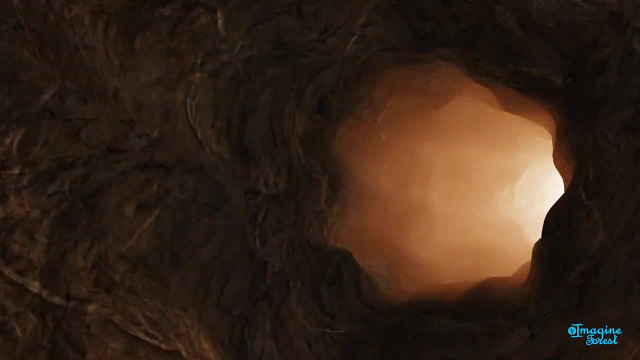 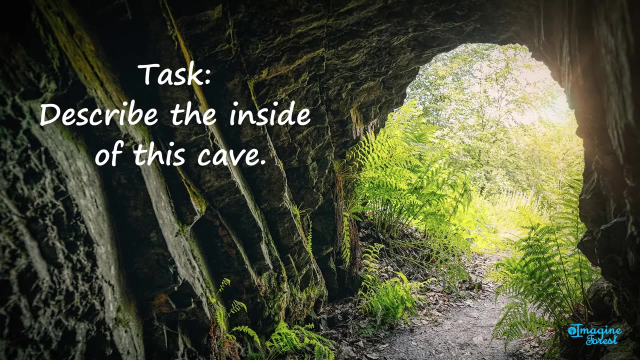 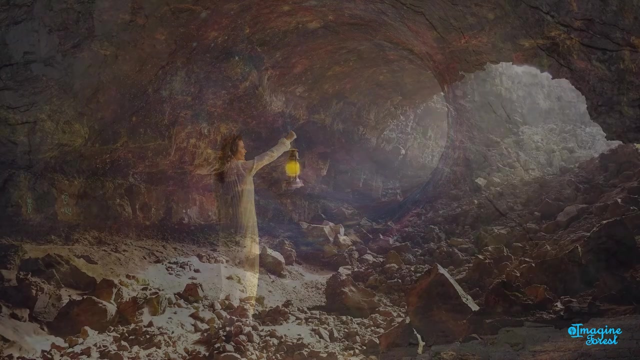 walk inside the cave, you see something very extraordinary. Your task is to describe what you see inside this cave. Here are some ideas to help you out. Think about the physical. Think about the physical appearance of the inside of this cave. Is it rocky and dark? 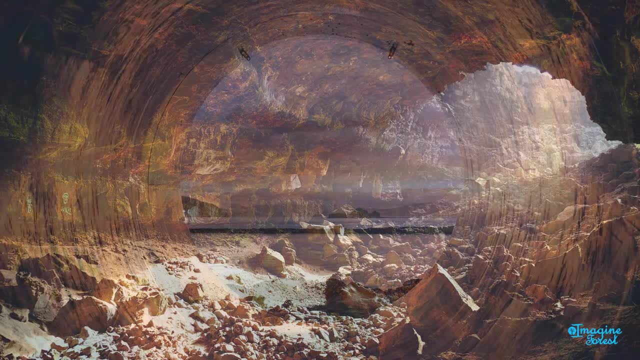 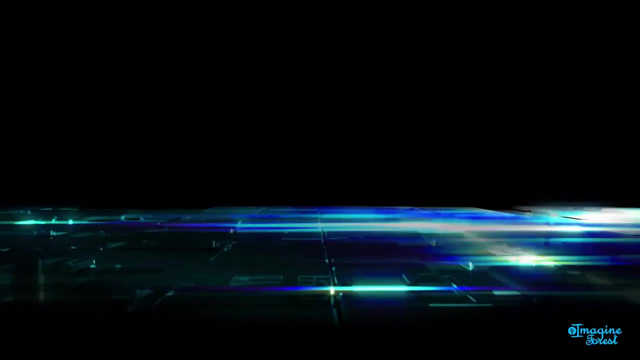 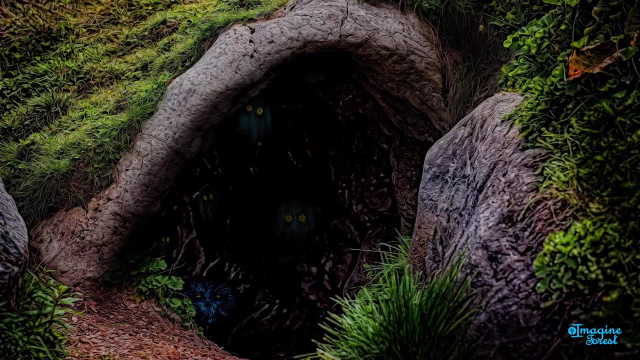 like a traditional cave, Or maybe it has golden walls, concrete columns and a glowing disco dance floor. Does anyone live in the cave and who lives here? Is it a cute, friendly bear Or is it a bear that lives in a cave? 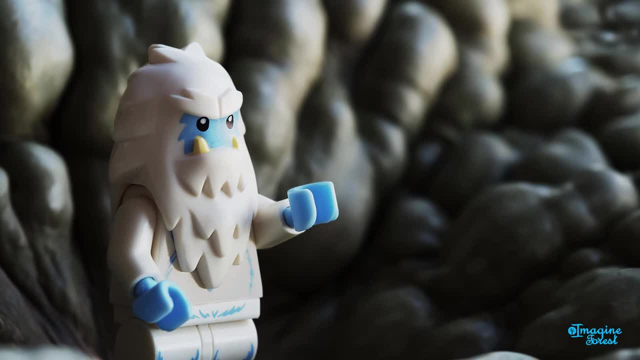 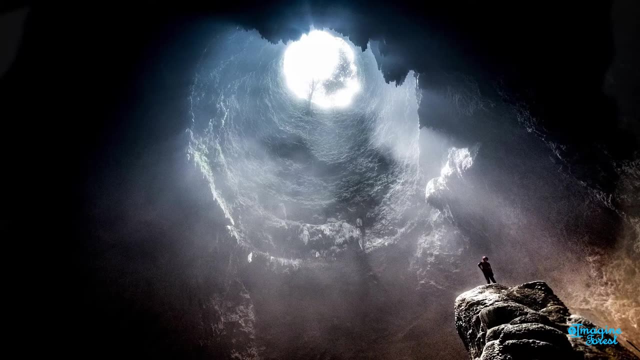 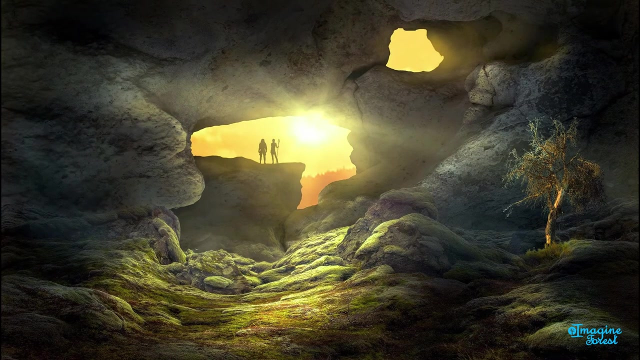 Or is it an evil, spiky monster who wants to eat you? Think about the way the cave smells from the inside. Does it smell of swamp water and freshly cut grass? Or maybe it smells of rotten eggs and stinky fish? 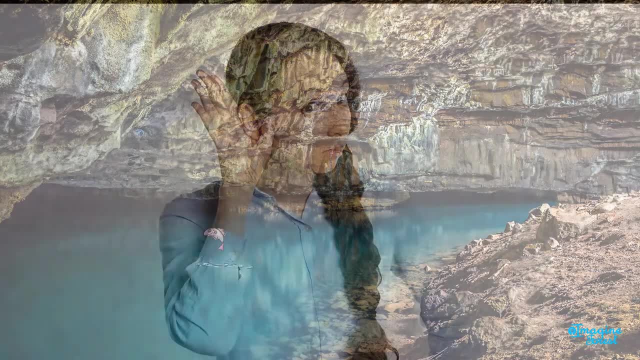 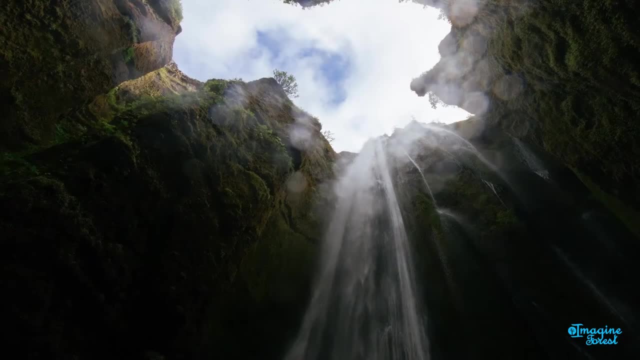 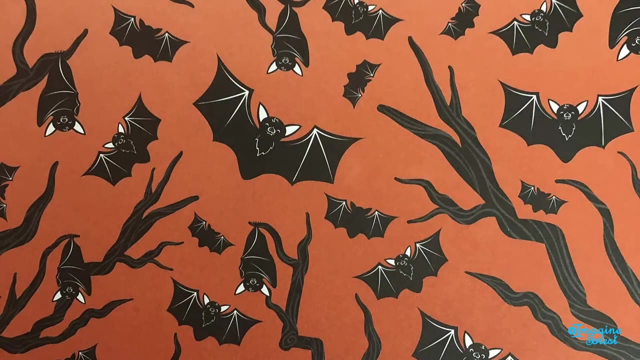 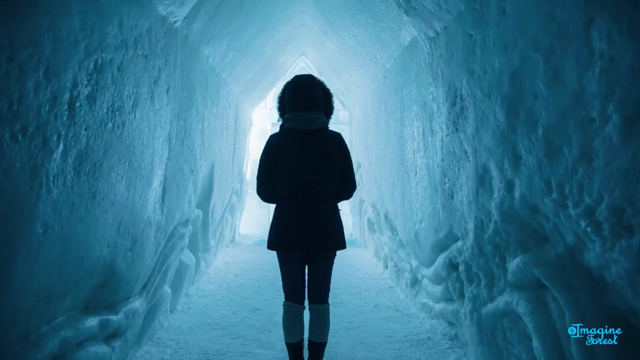 Use your ears. What do you hear as you enter the cave? Do you hear raindrops falling from the ceiling dripping downwards, Or maybe the sound of bats screeching in the distance? How do you feel as you enter the cave? Are you scared of what? 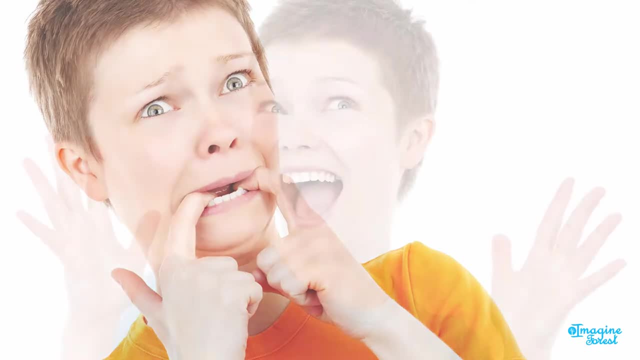